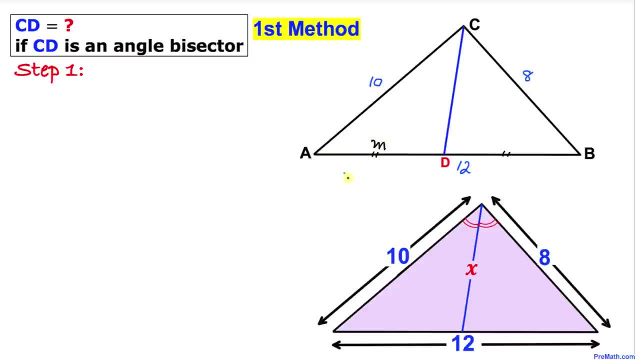 this AD, the length is going to be M, Then this DB is going to be: the total length, by the way of AB is 12, so DB is going to be simply 12 minus M. and here it is our angle bisector theorem. Here we have this proportion A over B. 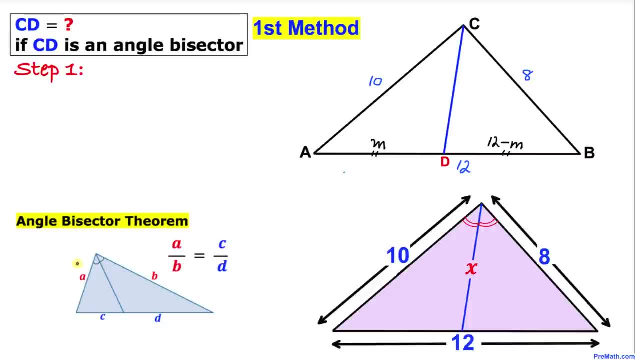 equal to C over D for this triangle that has these side lengths, AB, and then C and D. We are going to use this theorem in our this example. in this case we have A is 10, B is 8 and here C is our M and this D is our 12 minus M. Let's go ahead and apply that theorem. So we are going to. 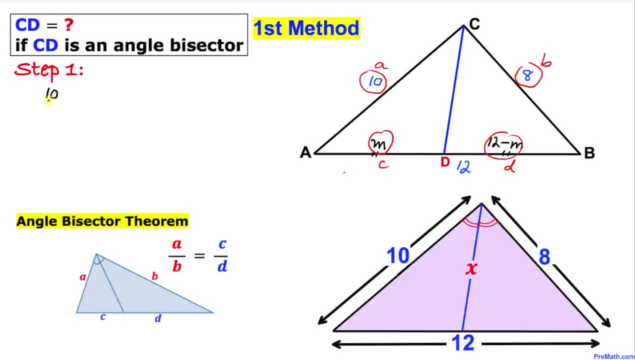 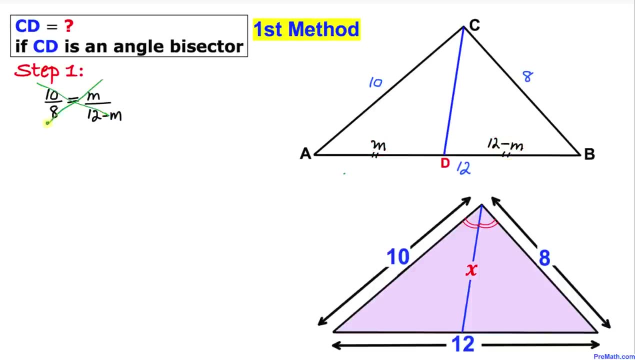 have A over B is going to simply become 10 over 8 equals to M over B. So we are going to have A over B is going to simply become 10 over 8 equals to M over B. Now let's go head and use a cross multiplication method to simplify. 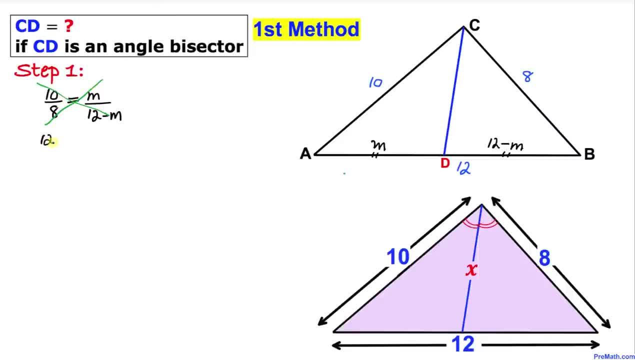 this one. so that is going to give us 120 minus 10 M equals to 8 M. Let's move this 10 M- the right hand side, so 120 equals to 8 M plus 10 M, which implies that 18 M equals to 120. let's isolate M by dividing both side by: 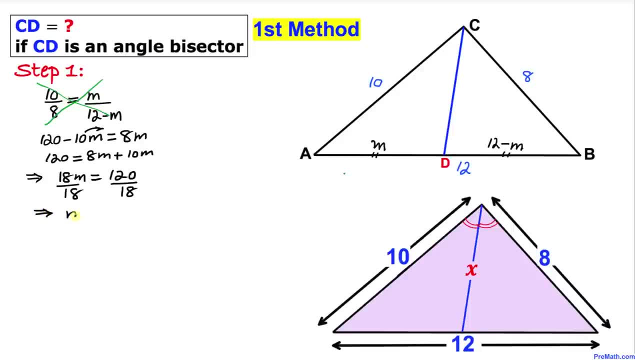 18. so that means M is going to be: if we reduce that one, that is going to give us 20 over 3. that is our M value. so that means this side AD, this segment AD, M equals to 20 over 3 and this DB is going to be simply 12 minus 20 over 3. and here 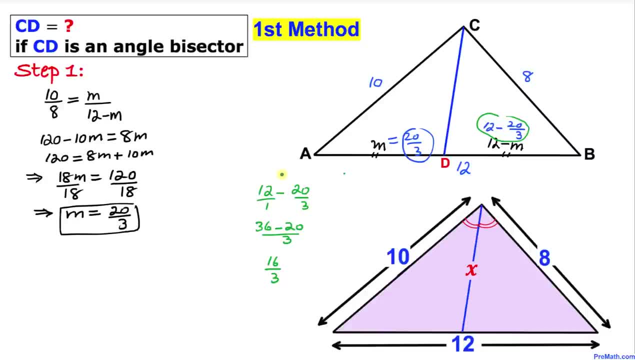 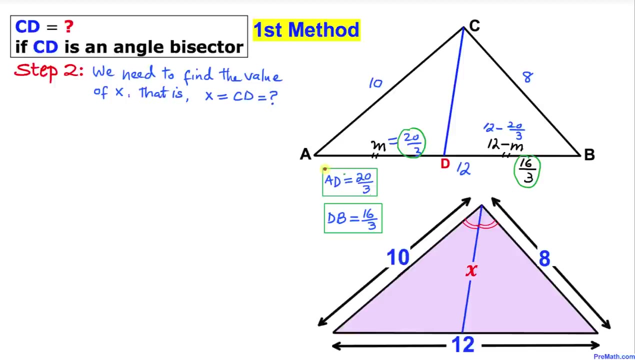 I have copied down this quantity right over here and I used crisscross method, cross multiplication, and this simplified into 16 over 3. so that means this DB side is going to be 16 divided by 3. and here's our next step. we are interested in finding the value of this. 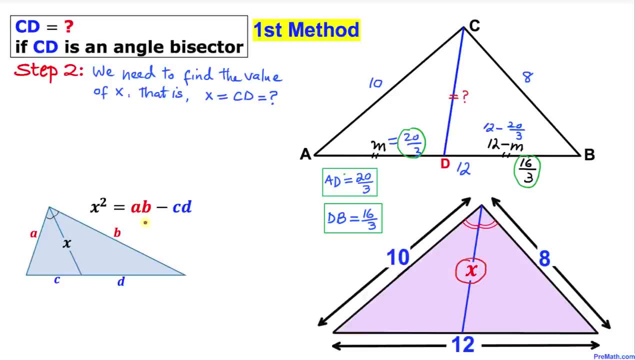 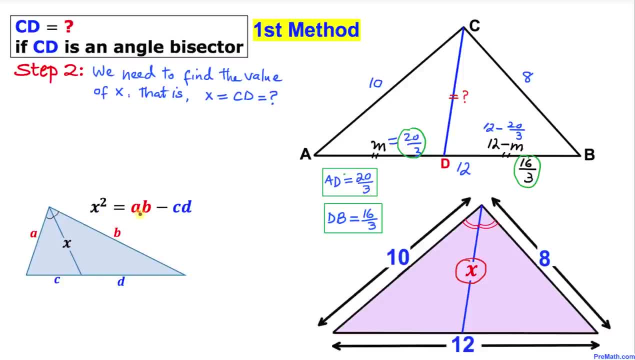 and this time we are going to calculate the value of the X value. let's go ahead and use this theorem to our this given problem. in our case, this 10 is our a. this 8 is our B. this value is our C. this 16 over 3 is our value D. 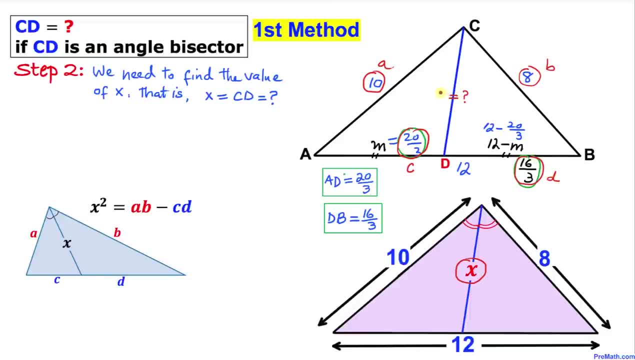 and this segment CD is our X. so let's go ahead and replace the value in this formula. so this is going to become x squared equal to a, in our cases 10 times 8 minus 20, divided by 3 times 16 over 3. let's simplify that one that is going to. 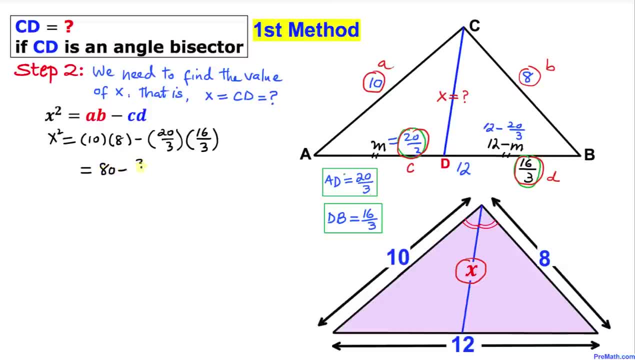 give us 80 minus 320 divided by 9, and if we simplify that thing, that is going to give us 720 minus 320 divided by 9. that is going to give us 400 divided by 9 is equal to x square. let's go ahead and take the square root on both side. 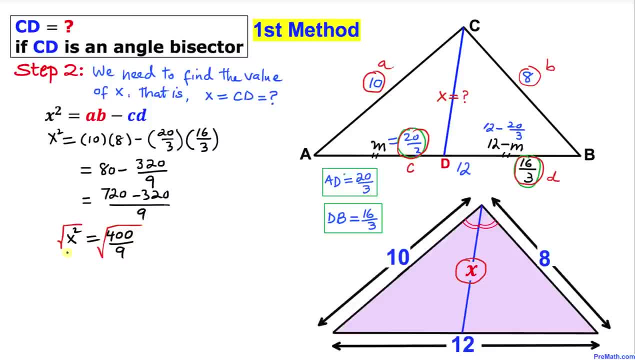 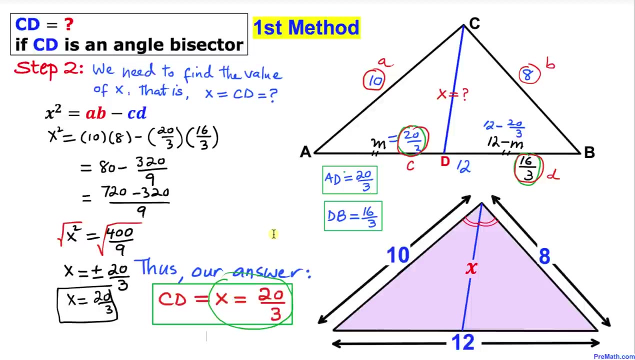 because we need X value. so we got X equal to positive or negative 20 over 3. so X is going to become positive 20 divided by 3. so that's, our X value turns out to be 20 divided by 3. and now I'm going to show you the second method, and it is called: 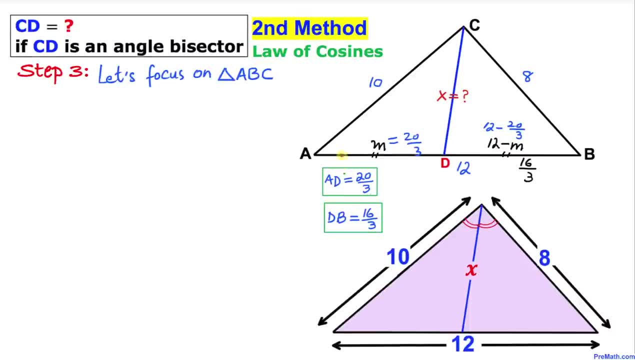 law of cosines. and now, in this next step, let's focus on this big triangle ABC, and let me go ahead and call this angle alpha, this angle alpha. and here is our law of a square equal to b square plus c square minus 2 times BC, cosine of alpha. and if we use this, 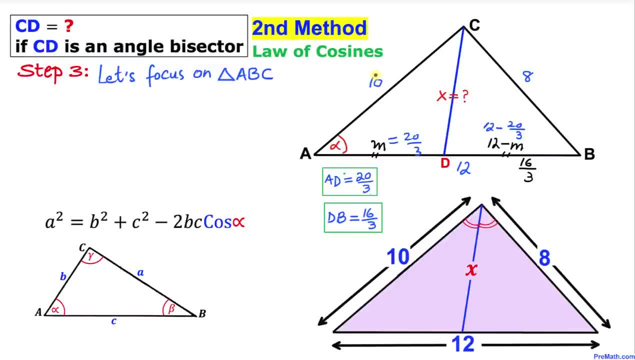 rule in our example. in this case, our a is going to be 8, this B is going to be 10 and this C is going to be 12, so let's go ahead and fill in the blanks in this cosines formula. so in our case a is 8, so it's going to become 8 square, and in our case, B is 10, so 10. 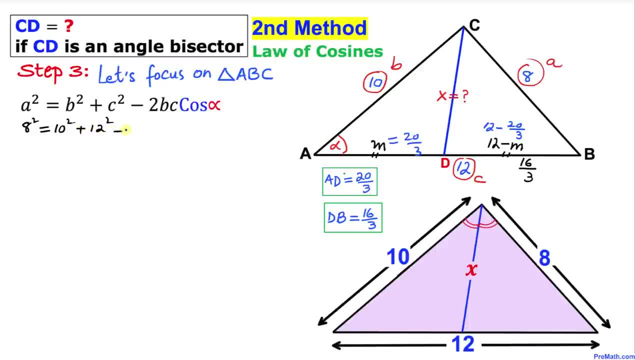 square plus C is 12 square minus 2 times 10 times 12 cosine of alpha. let's simplify 64 equal to 100 plus 144 minus 240 cosine of alpha. and let's simplify 64 equal to 140 cos sin of alpha. 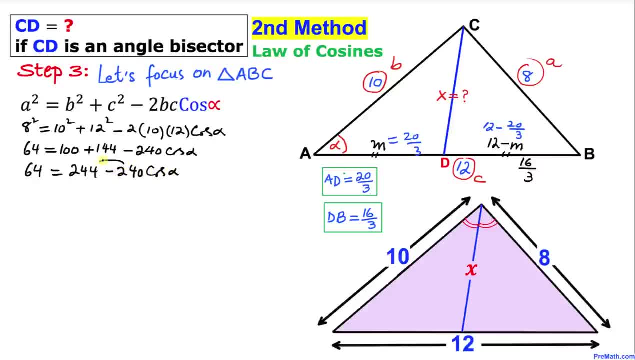 Now, third thing we need to see is that we need to see is that in Vedic heavens, the dwaivrts of физability is equal to b, and if we only talk about math and calculus of physics, it's going to Door to Qu í functioning. 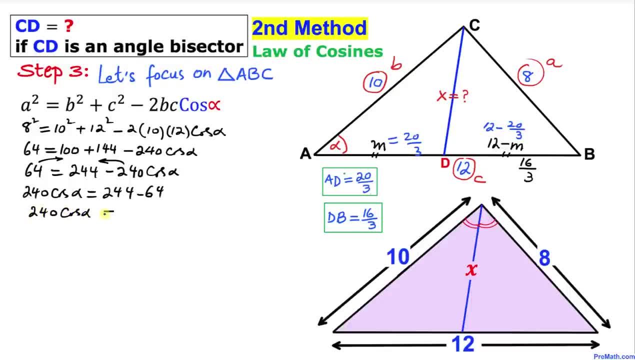 in馬ît, ведь мы looks like we have a complete network. We know that there is a equals 180. let's divide both side by 240 to isolate cosine of alpha. so that means cosine of alpha. if we reduce this thing, that is going to give us 3 over 4. so cosine of alpha turns out to 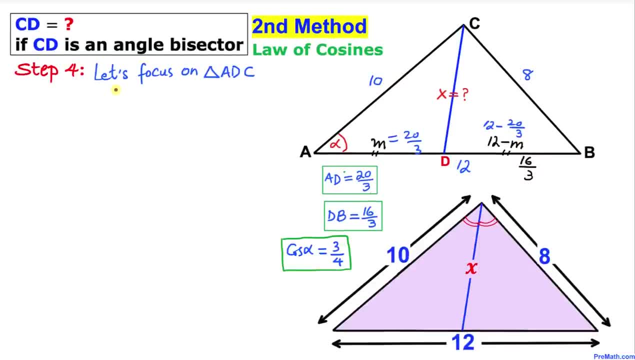 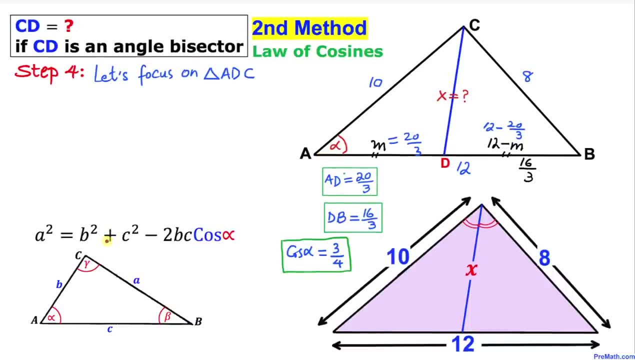 be 3 divided by 4. and here's our next step. let's focus this time on this triangle a, d, c, and here it is the law of cosines, once again, that we will be using in this problem again, and this time our a is going to be x, b is going to be 10 and our c is going to be 20 divided by. 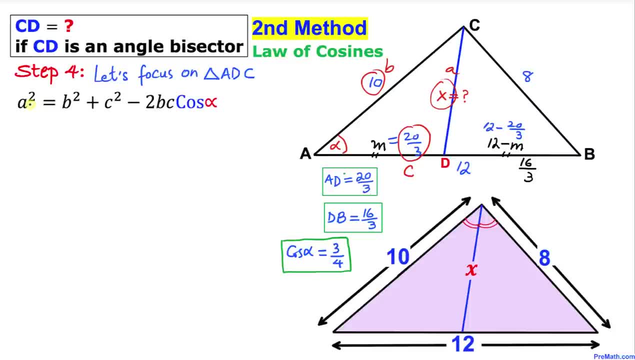 3. so let's go ahead and fill in the blanks in this law of cosines formula. in our case, a is x, so this is going to become x square equal to b. in our case is 10, so 10 square plus c is 20 divided by. 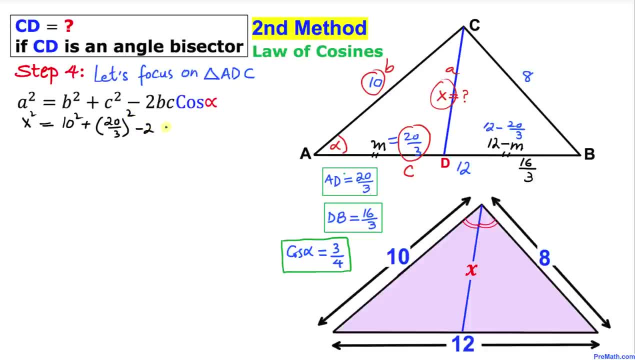 3 square minus 2 times 10 times 20, divided by 3 times cosine alpha. here we already figured out the value in our previous step. i'm going to replace it by 3 divided by 4. let's go ahead and simplify that one. so x square equal to 100 plus that is going to 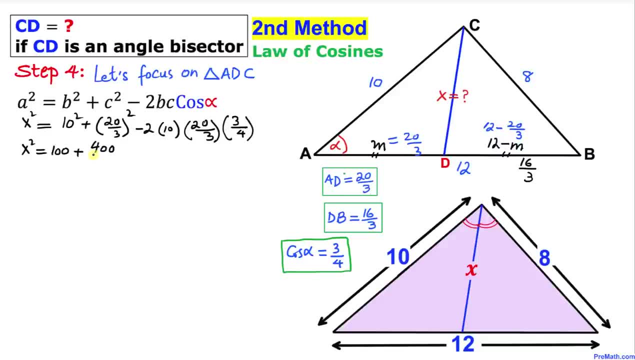 become 400 divided by 9 minus. that is going to give us- see, over here there's 3 and 3 is gone, so this 4 and 25 and that is going to give us negative 100. if we simplify and we can see that this positive and negative 100, they are gone. so we ended up simply x square equal to 400. 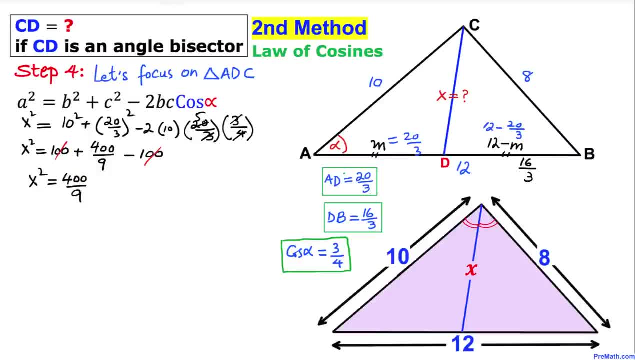 divided by 9. let's go ahead and take the square root on both side to undo this square. so this is going to be x square, equal to 4 and 3 is gone. so this 4 and 25 and that is going to give us.